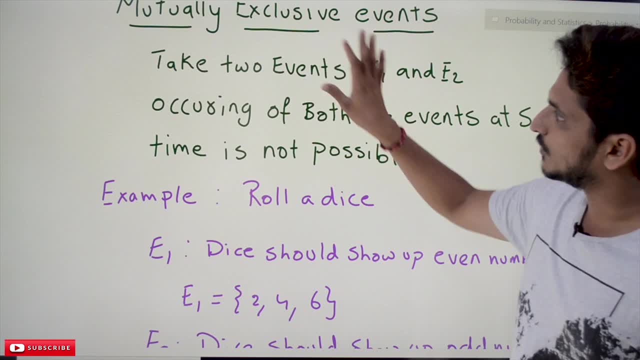 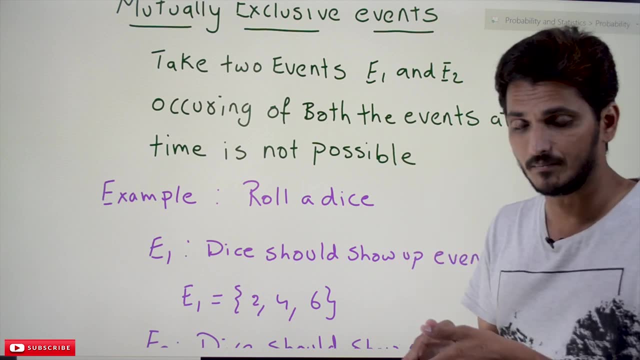 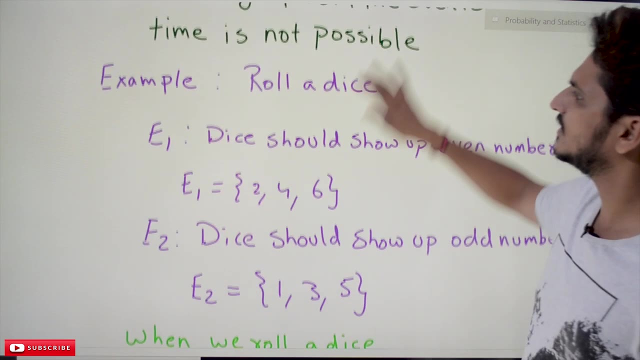 events which we are going to discuss in our coming classes. So make it clear here: mutually exclusive event means occurring of both the events at the same time is not possible. That is what we call. it is Mutually Exclusive Event. We will understand with an example, If you. 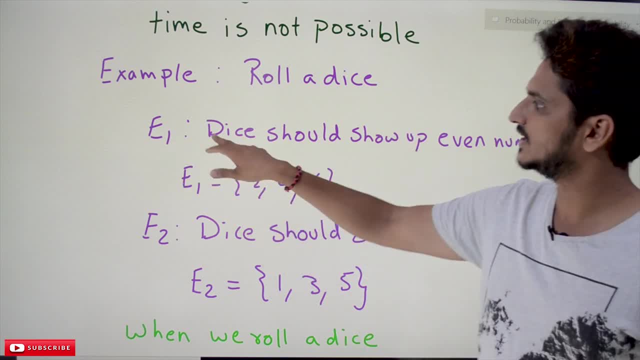 roll a dice And master the math. When you roll a dice, an event appears But DOUBLE E1.. End of the proves. E2 is epsilon white. E1 means tickish. the amount of some Missing eigenometric events at the same time is not possible In law. Mendel also defines E2 as an exponential event On the. 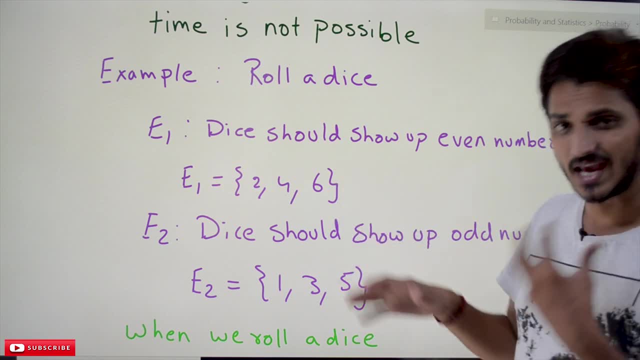 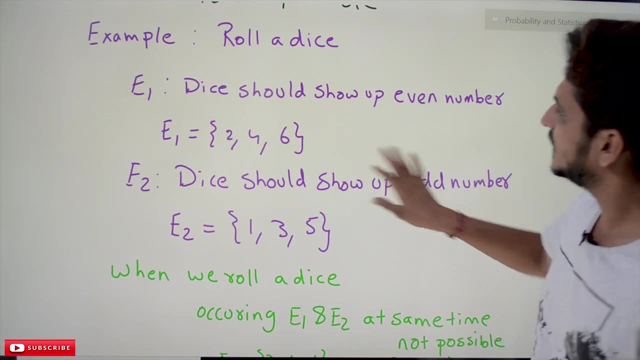 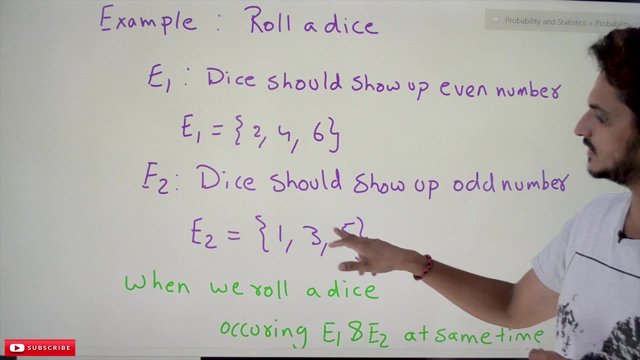 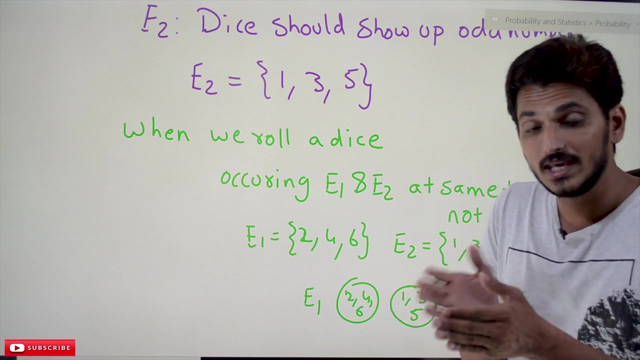 should show up even number. so what's the elements that present in the event? in the event, even even is equal to 2, 4, 6. if you take even t2 dice, show up odd number. what's the elements that present in e? 2 is 1, 3 & 5 if you take, if you roll a dice, when we roll a dice occurring of both the events. 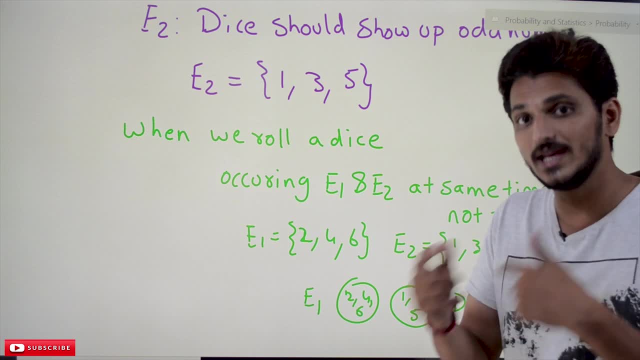 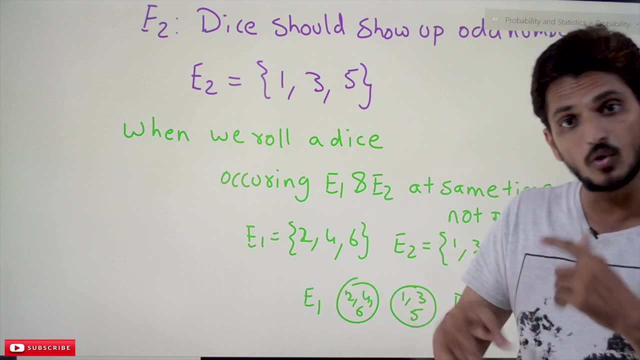 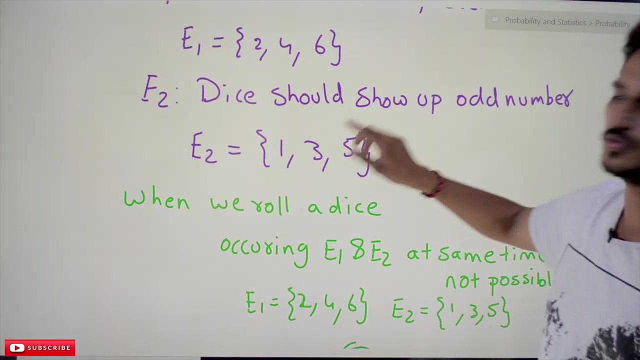 at the same time is not possible. that is what mutually exclusive events is. when we roll a dice, it may occur even number, it may occur odd number, but both, both is not possible. that is why these two events, even n Order, mutually exclusive events. so even is equal to four, six, eat is equal to one. 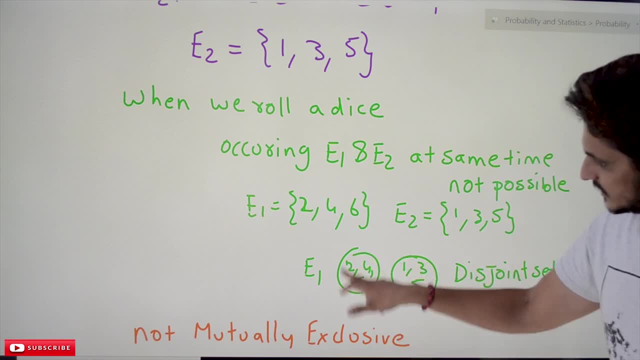 three, five, if you show it in that said, far matter said, even set consists of two, four, six elements. e two set consists of one wrap-around screen, three, five elements. these two sets are disjoint sets means they are not overlapping mutually exclusive event. sets are disjoint sets means intersection of these two sets is null, nothing. 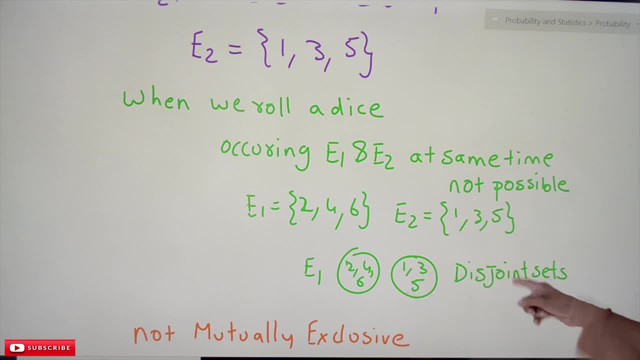 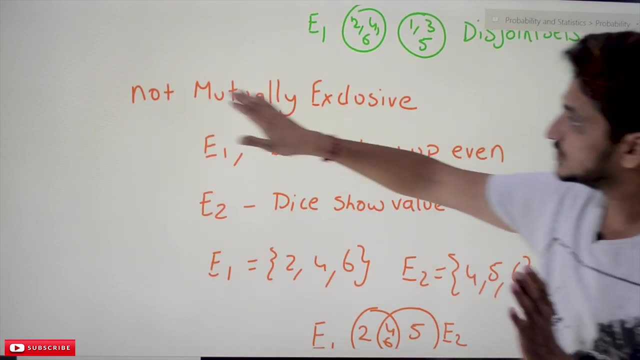 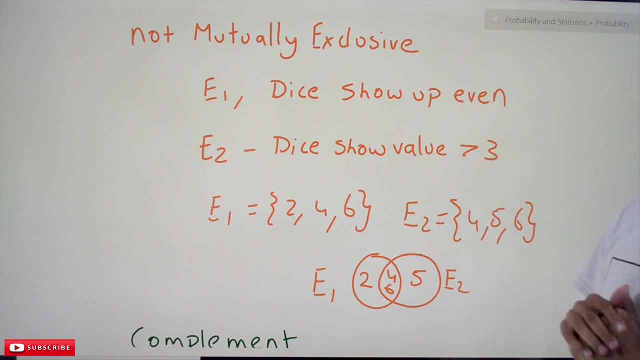 that's why we call it as disjoint sets this point also important to understand our coming classes. now, coming to one more example we will understand, which is not a mutually exclusive event. events even is equal to dice: show up even number. that is what we call it as event even. 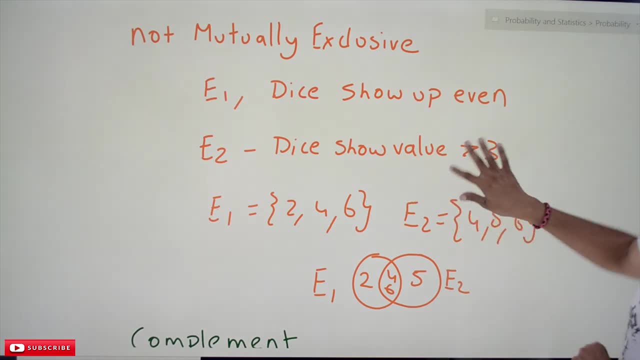 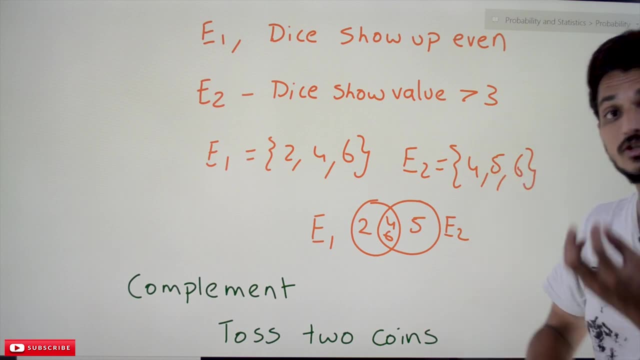 e2 is dice should show up value greater than 3. so what's the values? that is, 2, 4, 6 comes to e1. 4, 5, 6 comes to e2. when we roll a dice, it, if it show up 4, means it belongs to both. event 1: 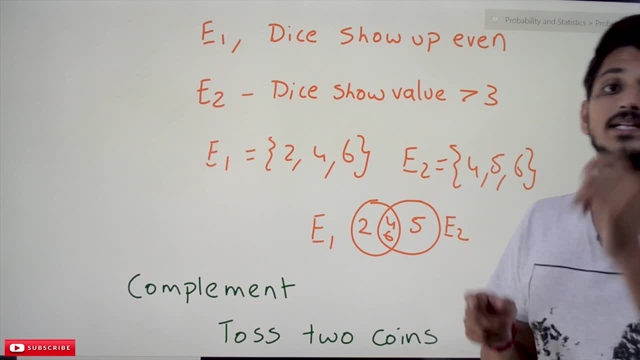 and event 2 occurring of both the events at the same time is not possible for mutually exclusive events. you here it is possible. that's why these two events are not mutually exclusive events. so 2, 4, 6 in the intersection part. if you show it in the set format, intersection part consists of 4, 6 and e2 consists. 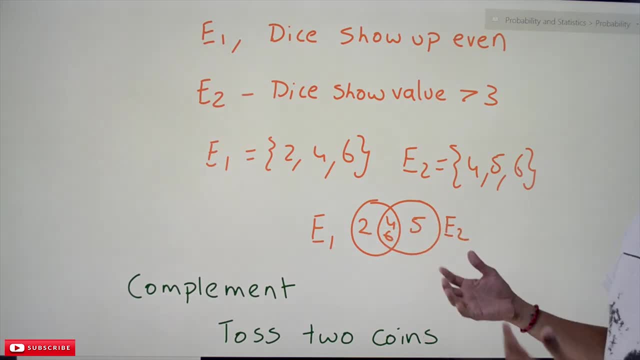 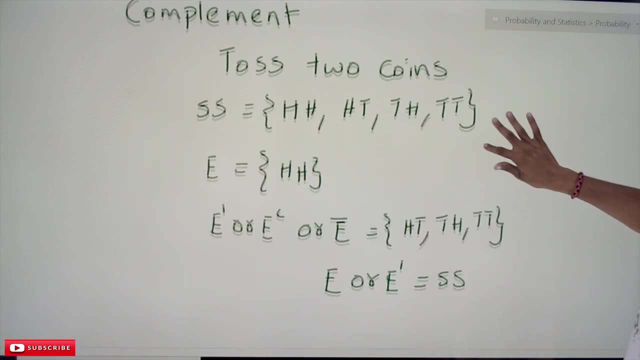 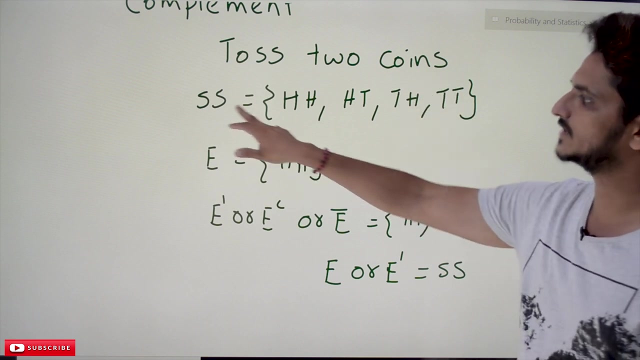 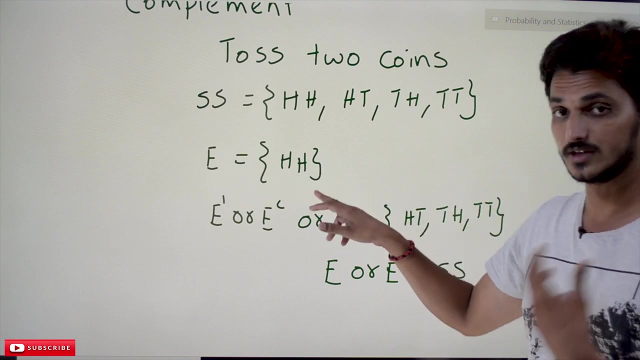 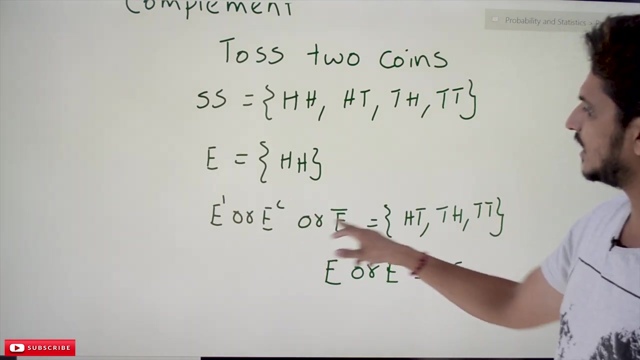 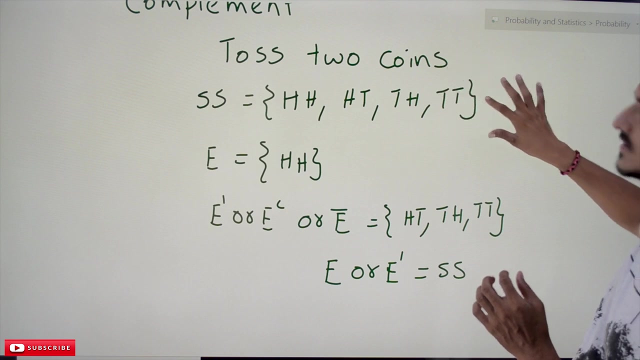 of 5, 5, 4, 6, 2, 4, 6, so these are not disjoint sets, overlap of two sets. now coming to the next one: complement, complement events- toss two coins. let's take an example and understand what's complement events means: toss two coins. sample space consists of head, head, head tail, tail, head, tail, tail. event e is equal to head head if you take, if you consider that event e is equal to head head. e complement is written like this: e dash or e complement or e bar the elements that are not belonging to e and that belong to the remaining sample space. remaining elements in the sample space comes under e. complement is written like this: e dash or e complement or e bar the elements that are not belonging to e and that belong to the remaining sample space. remaining elements in the sample space comes under e. complement is written like this: e dash or e complement or e bar the elements that are not belonging to e and that belong to the remaining sample space. remaining elements in the sample space comes under e. complement is written like this: e dash or e complement or e bar the elements that are not belonging to e and that belong to the remaining sample space. remaining elements in the sample space comes under. e complement is written like this: e dash or e complement or e bar the elements that are not belonging to e and that belong to the. 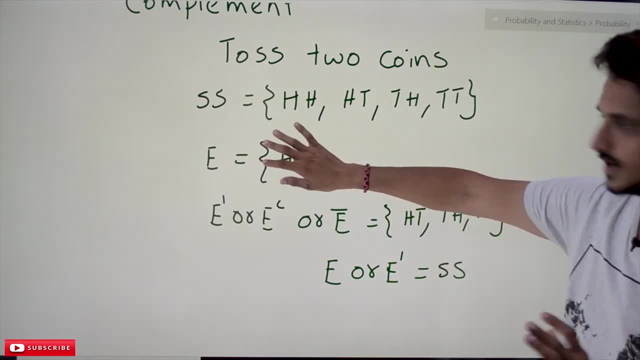 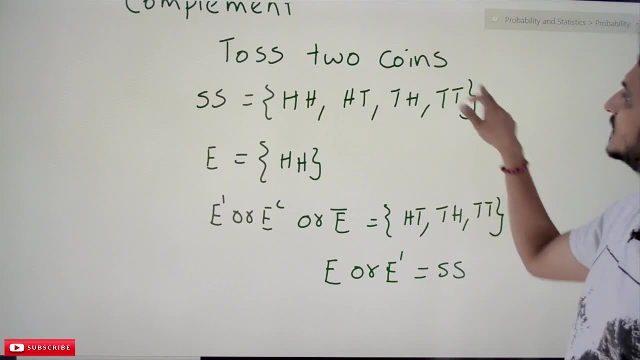 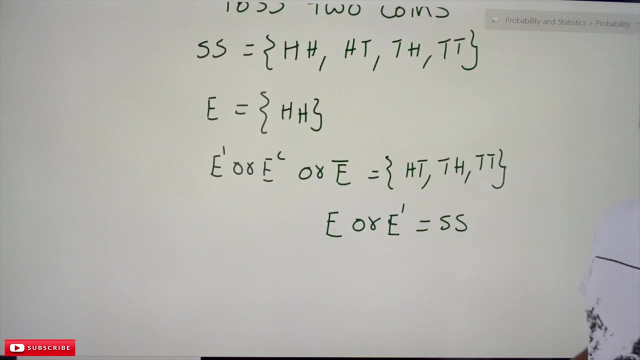 element. so head, head, belong to our event, the elements that belonging to the remaining elements in our sample space. so if you take it out, head, head, what's the remaining elements in our sample space? head, tail, tail, head, tail, tail- these comes under e complement. so e complement consists of head, tail, tail, head and tail tail. so one more important point you have to remember here: e or e complement. if you take e complement, e event, e are e complement. that 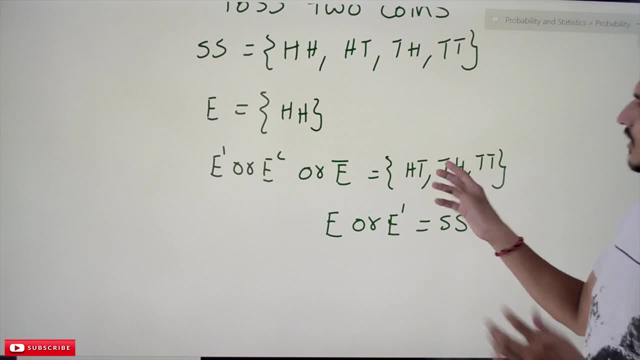 equal to sample space. Either this or that means entire sample space will come into existence. You can take an element that belongs to E, or you can take an element belongs to E. complement means it is sample space. This is about complement and mutually exclusive events. Hope you understand. 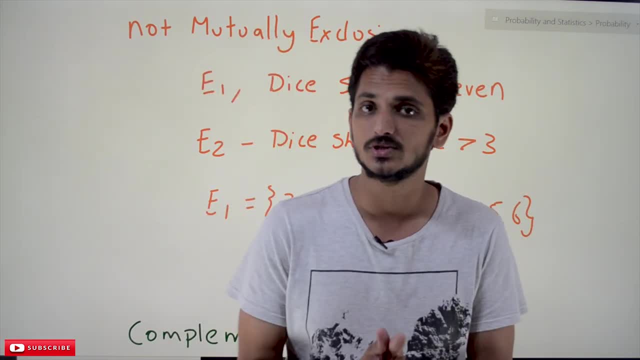 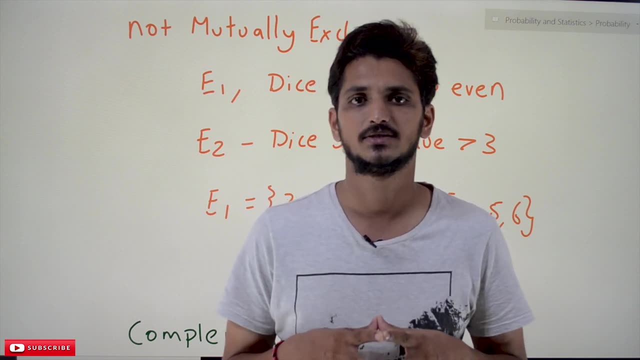 the concept. If you have any questions regarding the concept, please post your questions in the comment section below. Thanks for watching. If you haven't subscribed to our channel, please subscribe to our channel and press bell icon for the latest updates. Thank you.